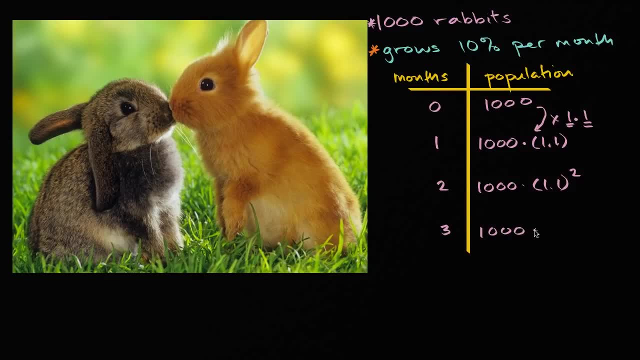 After another month, the population's gonna be 1,000 times 1.1 to the third power. We're just gonna multiply by 1.1 again, And so if you were to go n months into the future, well, you could see what's going to be. 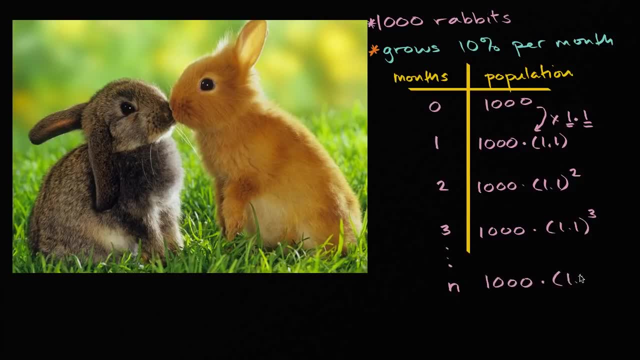 It's gonna be 1,000 times, or being multiplied by 1.1, n times, or 1,000 times 1.1 to the nth power, And so we can set up an expression here. We could say: look the population. 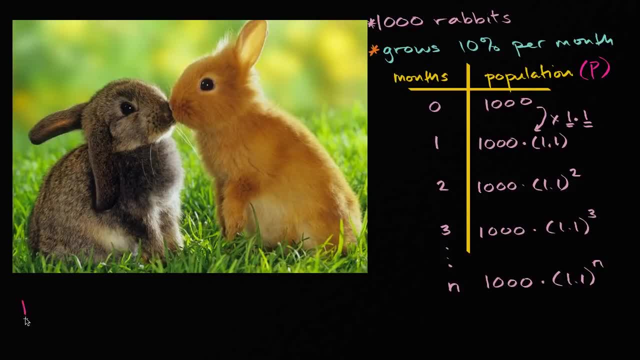 let's say that the population is p, The population as a function of n, as a function of n is going to be equal to our initial population, our, our initial population times 1.1 to the nth power. And you might say, okay, well, this makes sense. 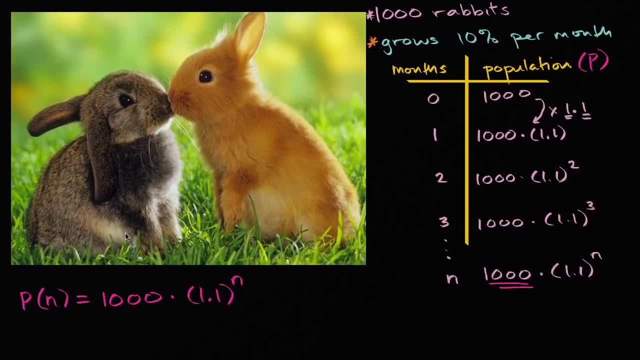 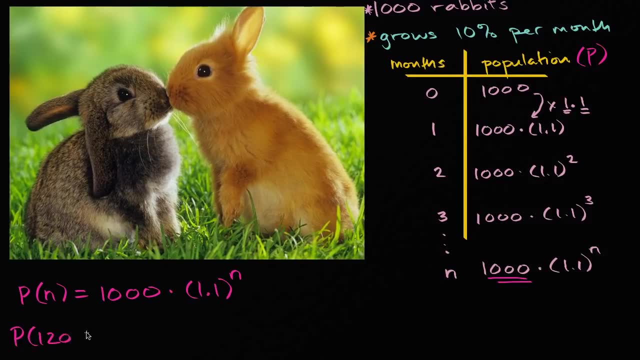 It doesn't look like we're getting crazy numbers, But just for kicks. let's just think about what's going to happen in 10 years. So 10 years would be 120 months. So the population at the end of 120 months. 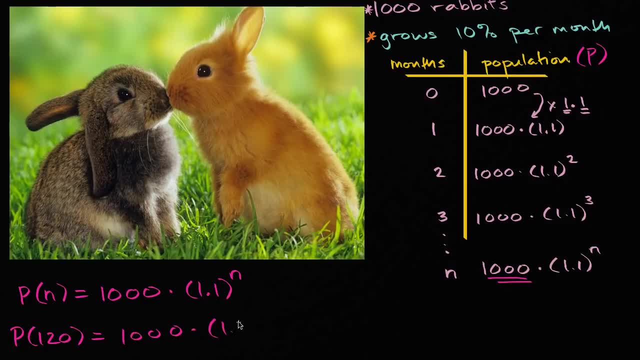 is going to be 1,000 times 1.1 to the 120th power, And so let's, let me get a calculator out to do that. I cannot calculate 1.1 to the 120th power in my head. 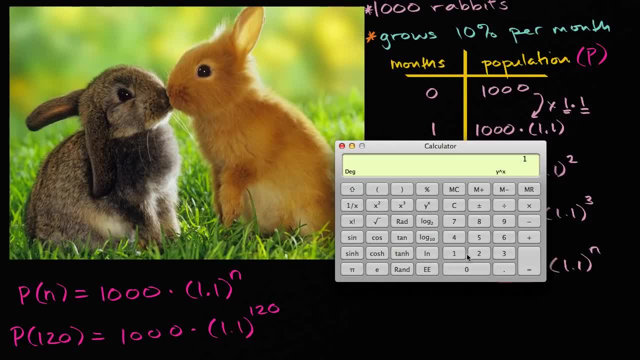 1.1 to the 120th. power is equal to that times our initial population, so times 1,000.. One, two, three Is going to be equal to roughly 93 million rabbits. Lemme, write that down. So we started with 1,000,. 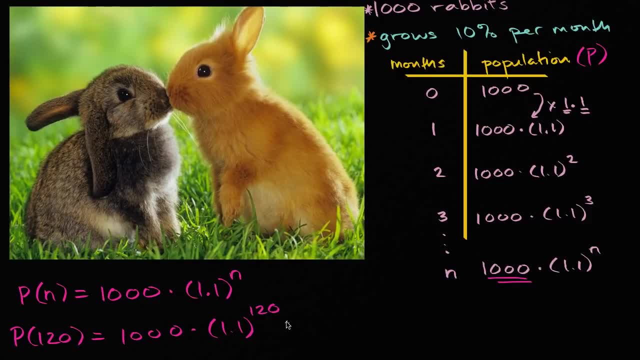 and we're going to have approximately 93 million rabbits. 93 million million rabbits, And so we grew by a factor of 93,000 over 10 years. so over another 10 years we'd grow by 93,000 times this. 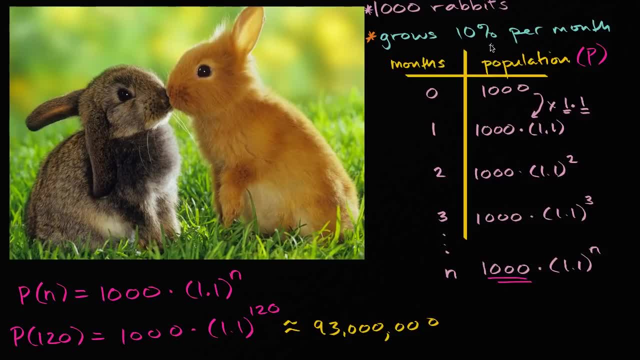 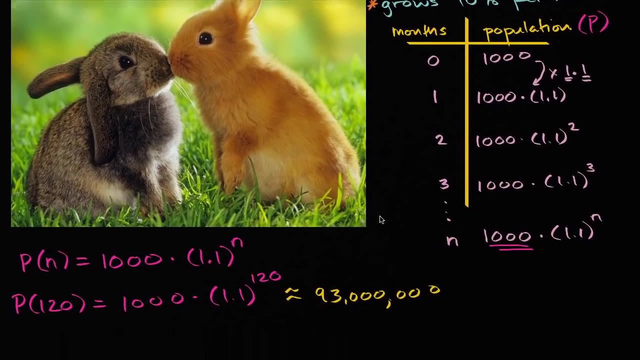 And so you quickly realize: 10% per month is quite fast And this might seem extremely fast, but this is actually not outlandish for a population of rabbits that are not limited by space or predators or food. And if you were to plot something like this out, 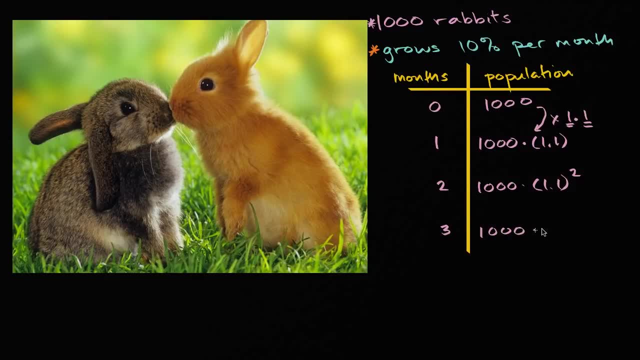 After another month, the population's gonna be 1,000 times 1.1 to the third power. We're just gonna multiply by 1.1 again, And so if you were to go n months into the future, well, you could see what's going to be. 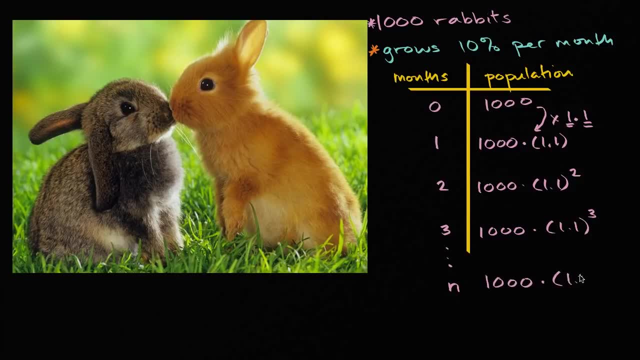 It's gonna be 1,000 times, or being multiplied by 1.1, n times, or 1,000 times 1.1 to the nth power, And so we can set up an expression here. We could say: look the population. 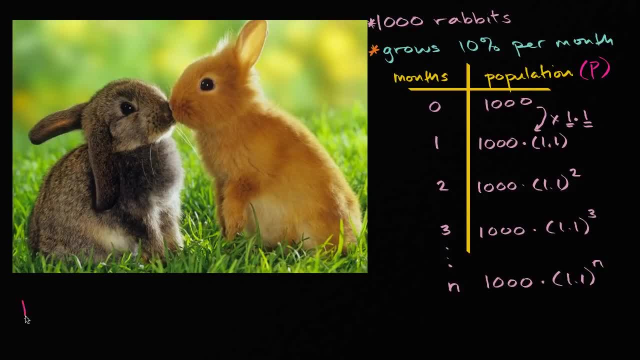 let's say that the population is p, The population as a function of n, as a function of n is going to be equal to our initial population, our initial population times 1.1 to the nth power. And you might say, okay, well, this makes sense. 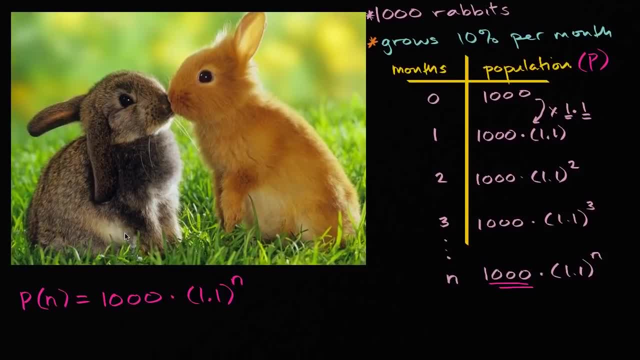 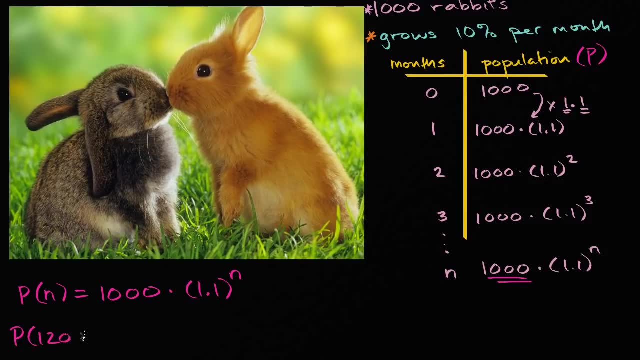 It doesn't look like we're getting crazy numbers, But just for kicks. let's just think about what's going to happen in 10 years. So 10 years would be 120 months. So the population at the end of 120 months. 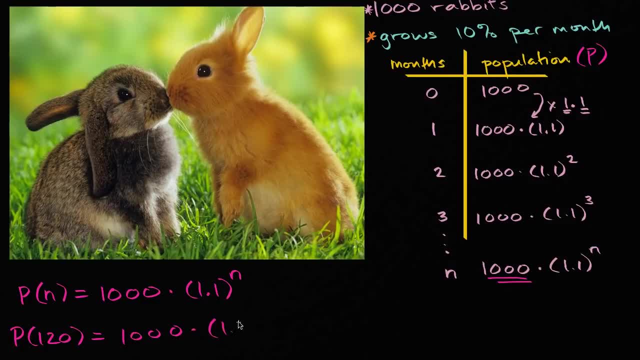 is going to be 1,000 times 1.1 to the 120th power, And so let's, let me get a calculator out to do that. I cannot calculate 1.1 to the 120th power in my head. 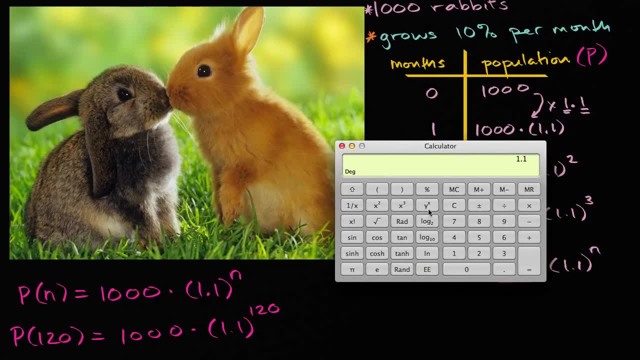 1.1 to the 120th. power is equal to that times our initial population. so times 1,000, one, two, three is going to be equal to roughly 93 million radicals Rabbits. let me write that down. 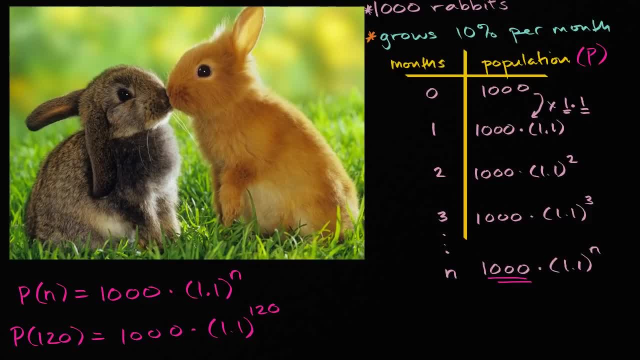 So we started with 1,000, and we're going to have approximately 93 million rabbits. 93 million million rabbits, And so we grew by a factor of 93,000 over 10 years. So over another 10 years we'd grow by 93,000 times this. 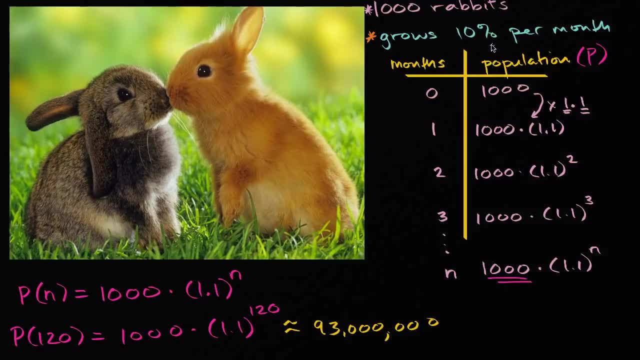 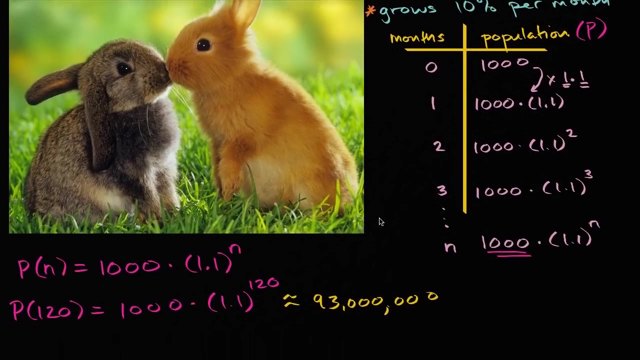 And so you quickly realize: 10% per month is quite fast And this might seem extremely fast, but this is actually not outlandish for a population of rabbits that are not limited by space or predators or food. And if you were to plot something like this out, 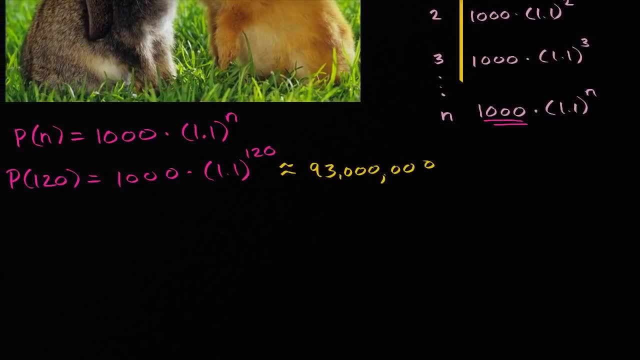 if you were to plot the rabbit population with respect to time, you would see a graph that looks. let me draw it. So this axis it is time, say in months, In this axis you have your population, You have your population. 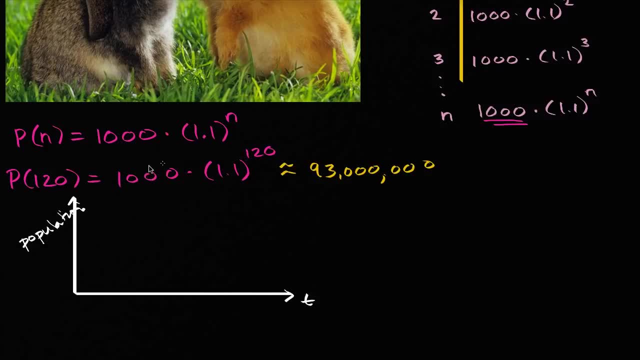 This type of function or this type of equation. let me see population. population, this is an exponential function, And so your population, as a function of time, is going to look like this. It's going to have this kind of hockey stick J shape. 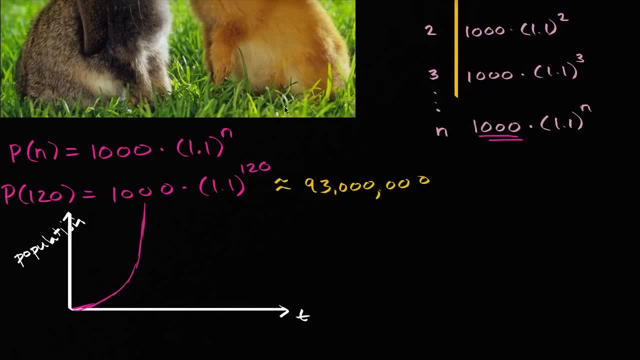 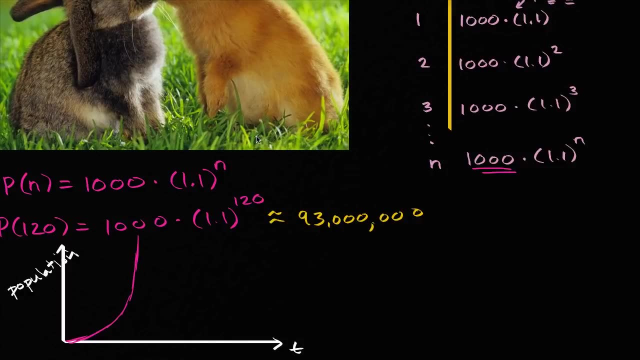 right over here And if you let these rabbits reproduce long enough, they would, frankly, take over the planet if they had enough food and if they had enough space to do it. But, as you notice, I keep saying if they have enough food and if they have enough space. 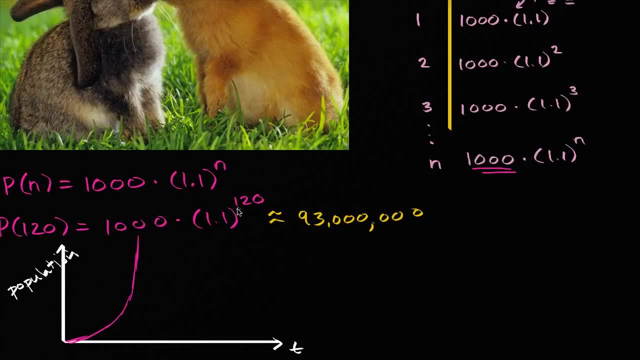 The reality in the world is that there is not infinite food and infinite space, and there are no, and it isn't the case that there are no predators or competition for resources, And so there is actually a maximum carrying capacity for a certain part of the environment. 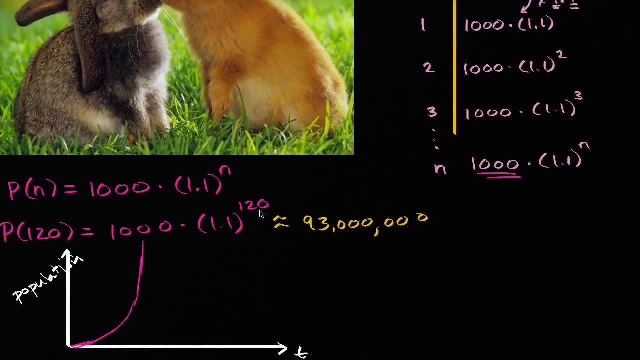 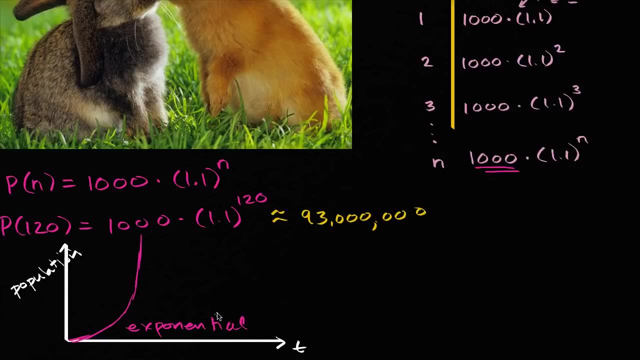 for a certain type of species, And so what's more likely to happen, what we just described right over here, is exponential growth. Exponential growth, And why is it called exponential growth? Well, you notice, we are growing by the input, which is time, is being thrown into our exponent. 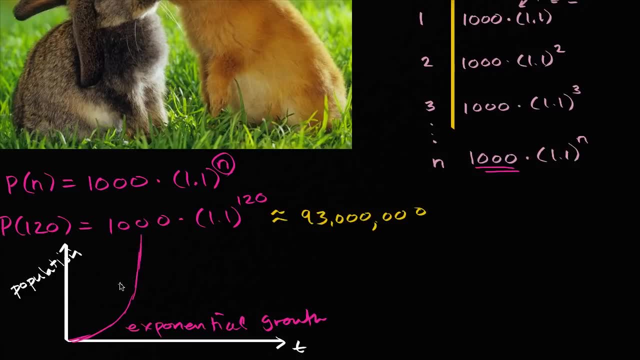 And so that is exponential growth. but obviously you can't have an infinite number of rabbits or you just can't grow forever. There is going to be some natural maximum carrying capacity that the environment can actually sustain And so the actual growth that you would see. 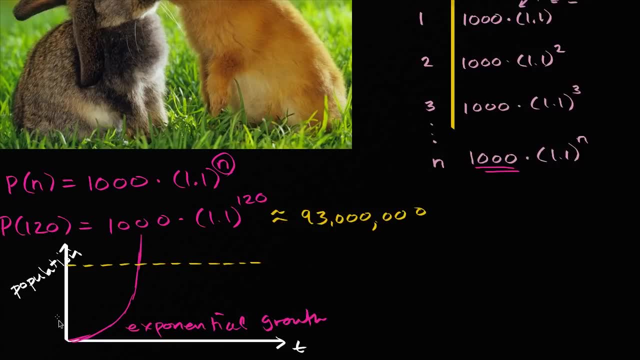 when the population is well below that carrying capacity, it's reasonable to model it with exponential growth. But as it gets closer and closer to that carrying capacity it is going to asymptote up towards it. So it's going to get up towards it but not cross it. 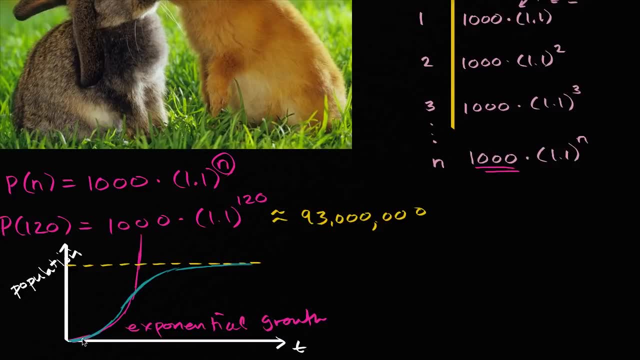 And that's just a model. There are other situations where maybe it goes up to it and it crosses it and then it cycles around it. So these are all different ways of thinking about it, But the general idea is you wouldn't expect something to just grow unfettered forever. 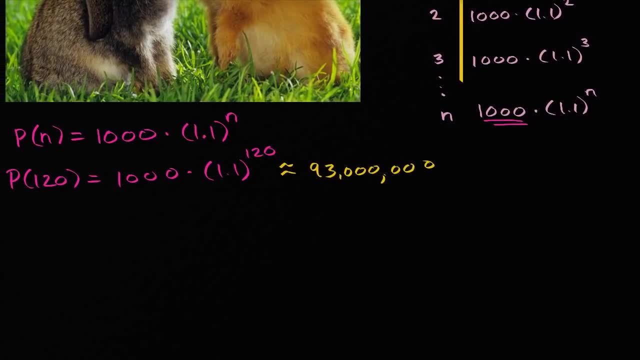 if you were to plot the rabbit population with respect to time, you would see a graph that looks. let me draw it. so this axis it is time, say in months, and this axis you have your population, you have your population. 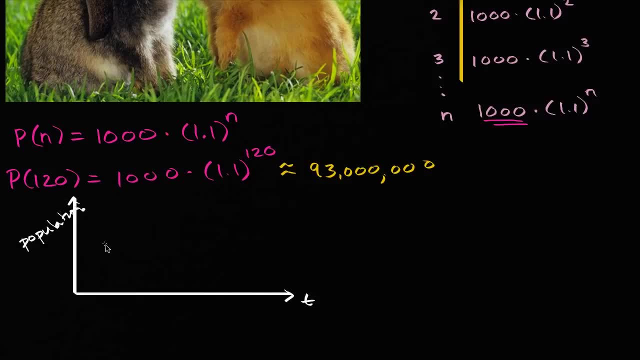 This type of function or this type of equation. let's see population: I, population. This is an exponential function, And so your population, as a function of time, is going to look like this. It's going to have this kind of hockey stick. 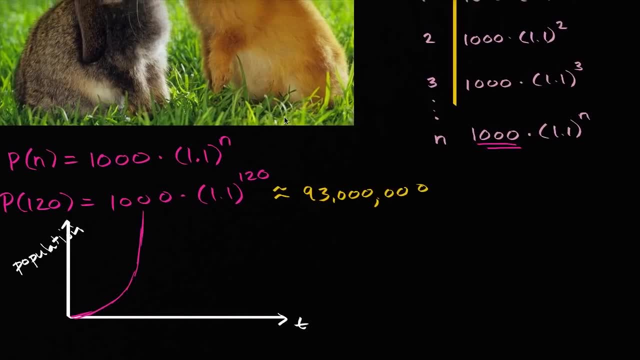 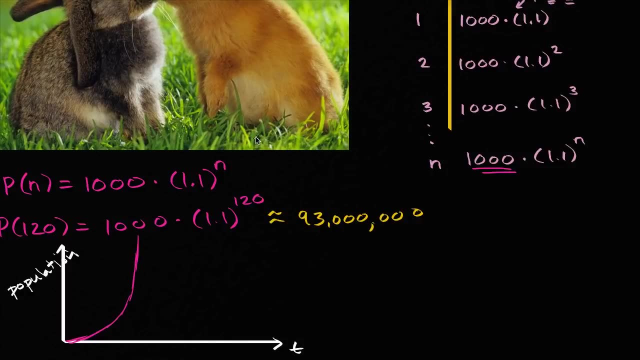 J shape right over here, And if you let these rabbits reproduce long enough, they would, frankly, take over the planet if they had enough food and if they had enough space to do it. But, as you notice, I keep saying if they have enough food and if they have enough space. 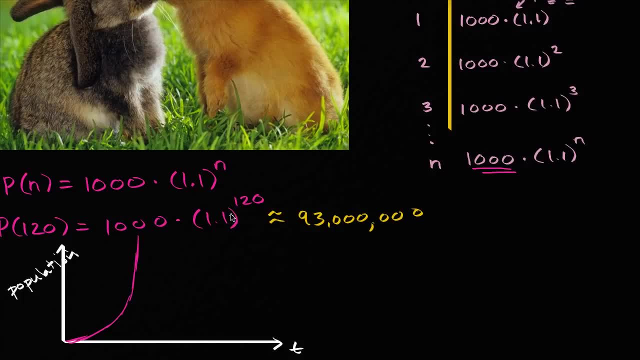 The reality in the world is that there is not infinite food and infinite space, and there is not and there are no, and it isn't the case that there are no predators or competition for resources, And so there is actually a maximum carrying capacity for a certain part of the environment. 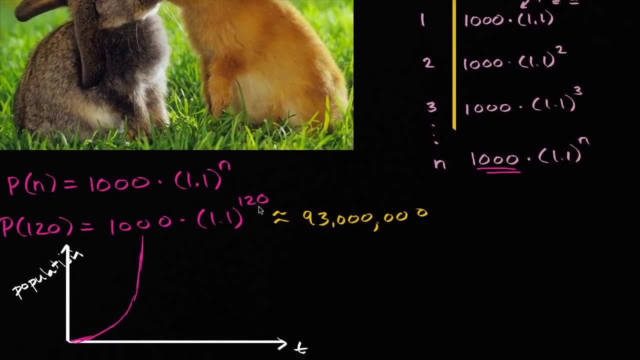 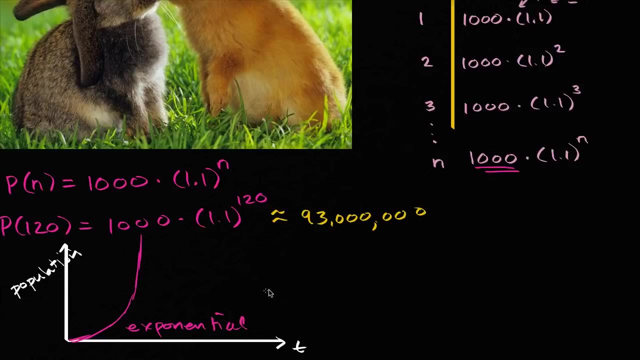 for a certain type of species, And so what's more likely to happen, what we just described right over here, is exponential growth. Exponential growth, And why is it called exponential growth? Well, you notice, We are growing by the input, which is time. 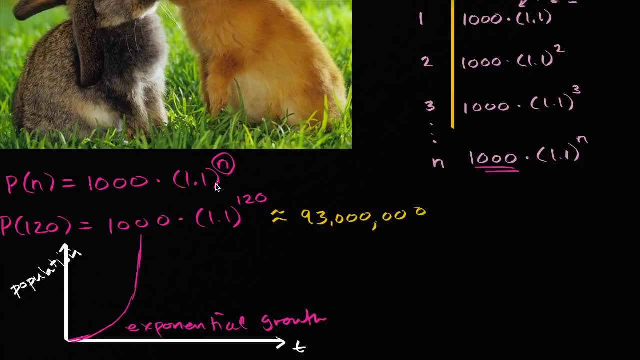 is being thrown into our exponent, And so that is exponential growth. but obviously you can't have an infinite number of rabbits or you just can't grow forever. There is going to be some natural maximum carrying capacity that the environment can actually sustain. 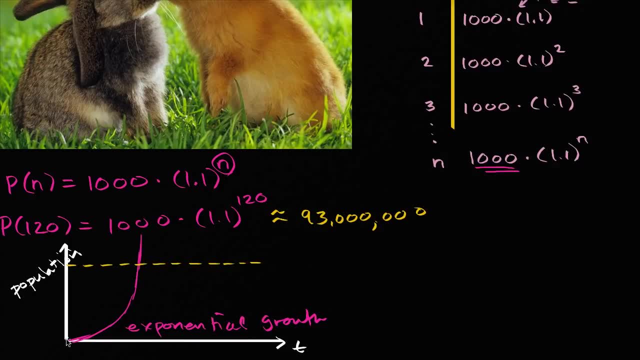 And so the actual growth that you would see. when the population is well below that carrying capacity, it's reasonable to model it with exponential growth. But as it gets closer and closer to that carrying capacity it is going to asymptote up towards it. 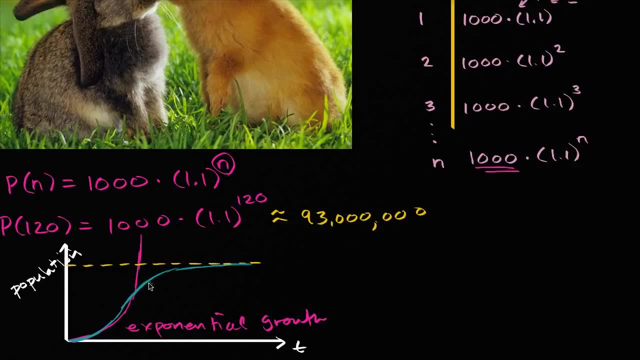 So it's going to get up towards it but not cross it, And that's just a model. There are other situations where maybe it goes up to it and it crosses it and then it cycles around it. So these are all different ways of thinking about it.